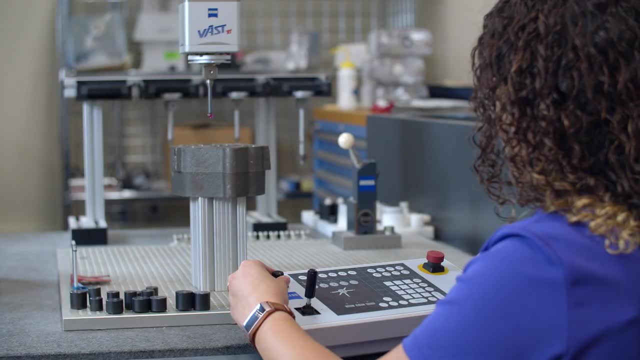 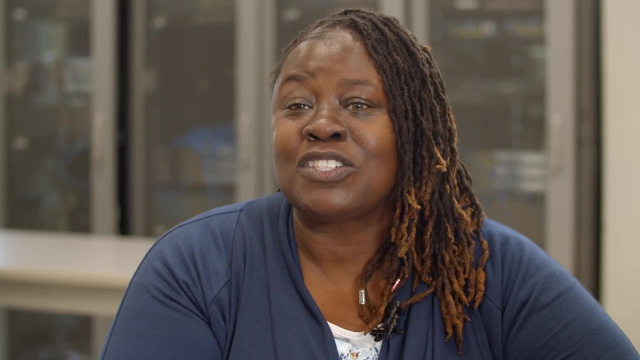 We do have our industry board working with us now on project management. We offer that in our departments and in project management they're actually going to be working with our students and mentoring so they can get their PHPs. So we divide engineering. 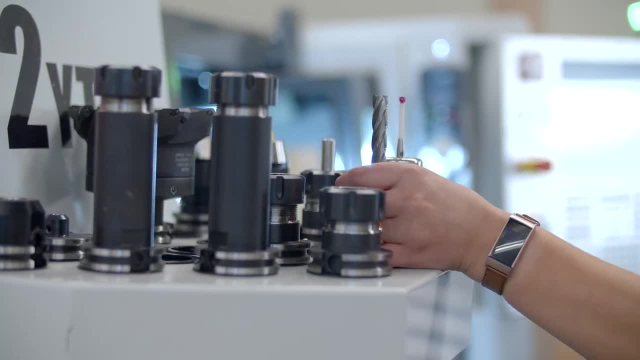 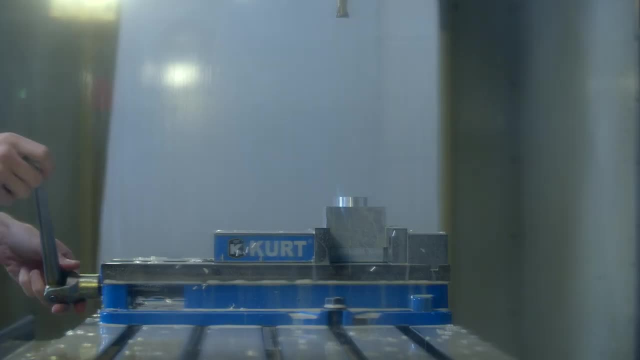 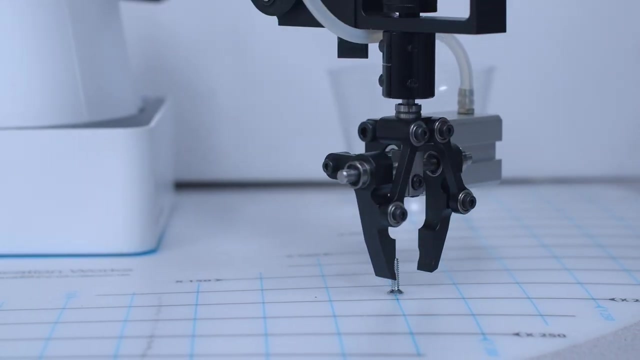 engineering technology into disciplines Electrical, mechanical, civil, chemical, automotive and many, many more. ET is a newer discipline. It came about because engineers were more involved with abstract problems. They would dive deep. In engineering technology you don't stand like a robot and push buttons. You design the robots. 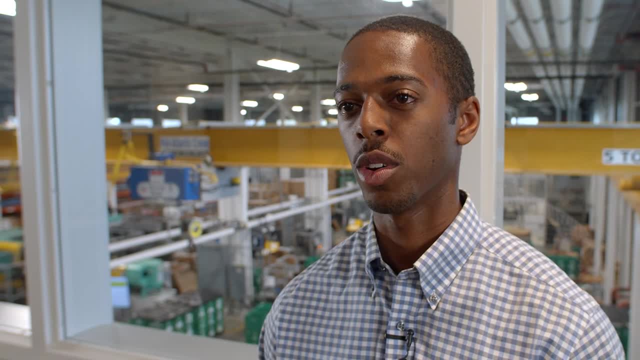 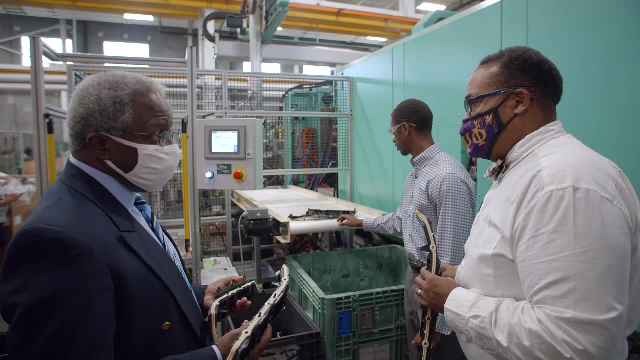 During my studies at A&T for engineering technology, I was given a high-level overview of manufacturing. I was then able to take that and apply that to the real world here at Cort Technology. I got this opportunity because one of my professors introduced me to the owner of the company. 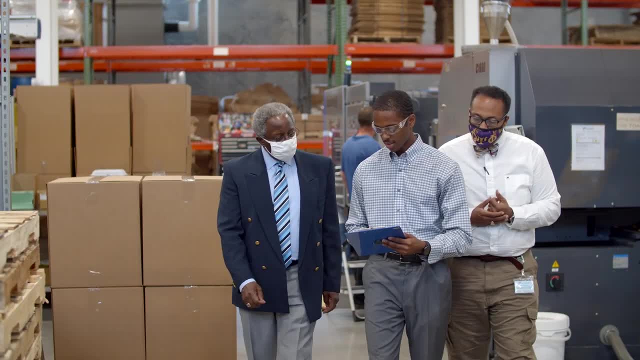 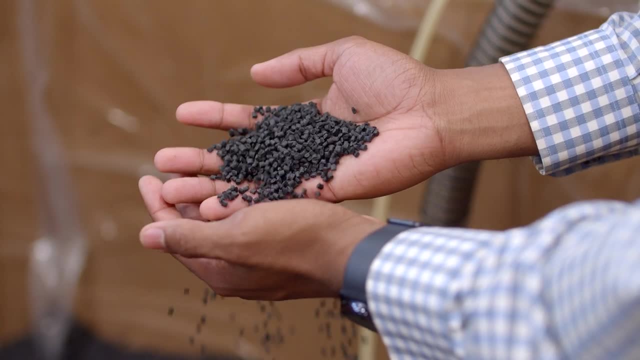 who then extended an offer for an internship. He, in fact, is also a graduate from the department I plan to work here at Cort Technology. I'll be graduating here in May, so I plan on working here full-time as a design engineer. 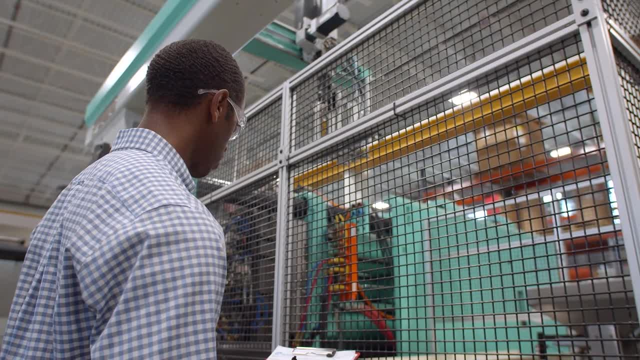 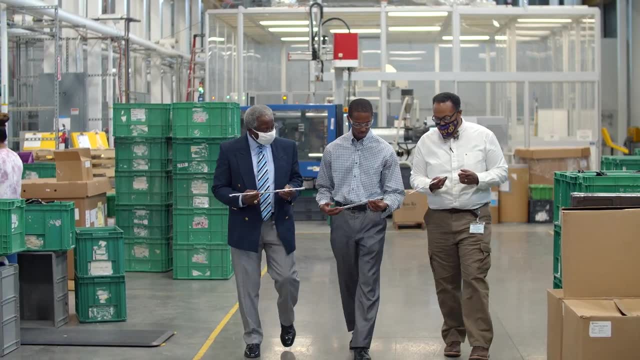 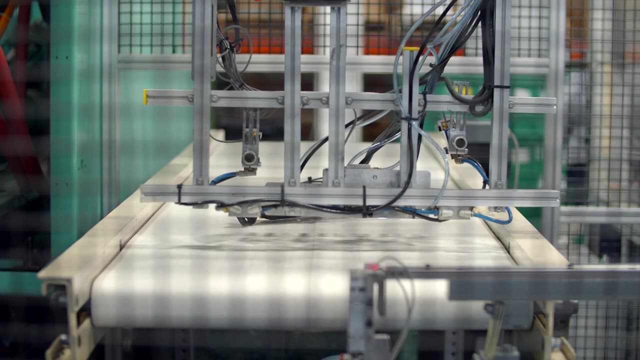 You can focus on design or manufacturing or you can find your own path. Teamwork is critical to success. We work with people. As part of a team, we can make things happen. Get to work with modern technologies. Do things that make a difference. 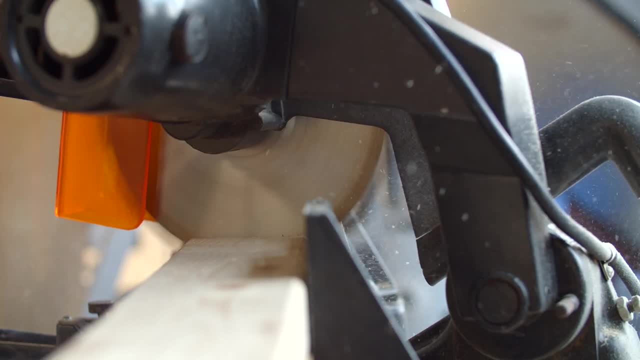 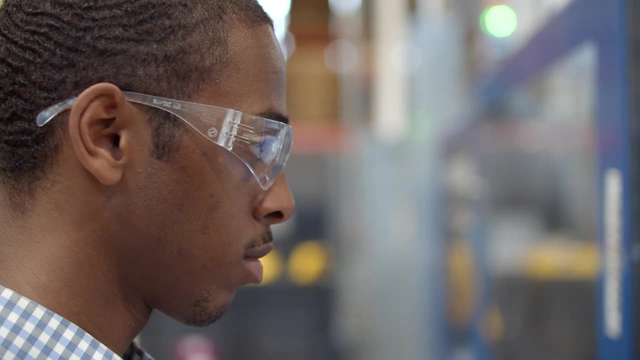 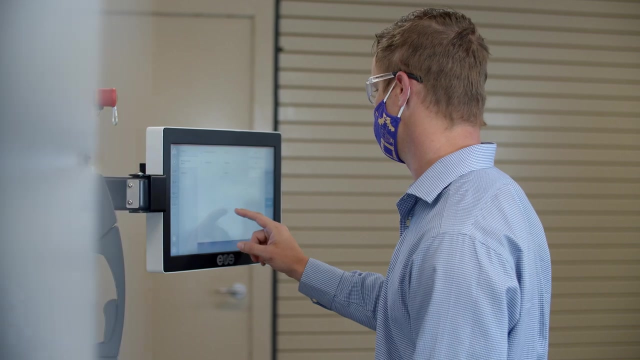 Innovation is key. We are professional inventors. There's a place for you here with us in engineering technology. Bring your ideas, Bring your hopes and ambitions. We'll help you realize your dreams. The only thing that will limit your career is your imagination. 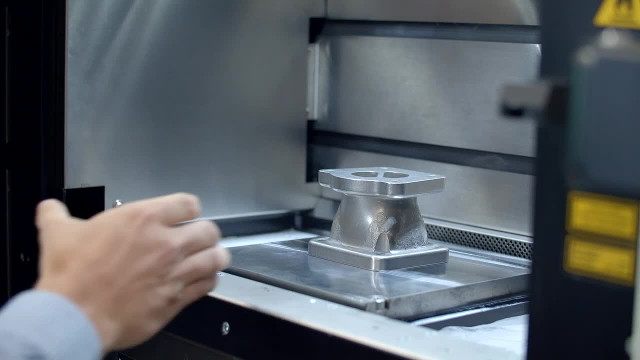 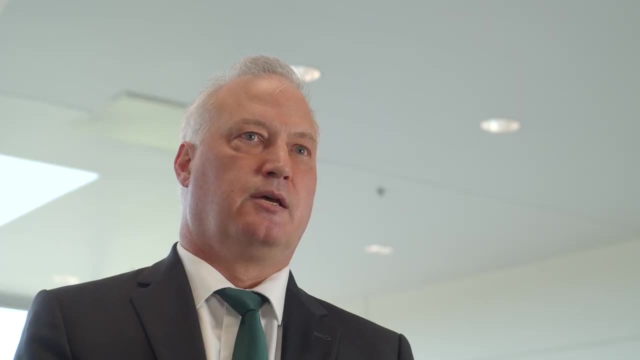 You can go where you want, when you want, with an ET degree. This video gives you a taste of some of the engineering technology disciplines. There are many more resources online. You can follow the link at the end of this video. 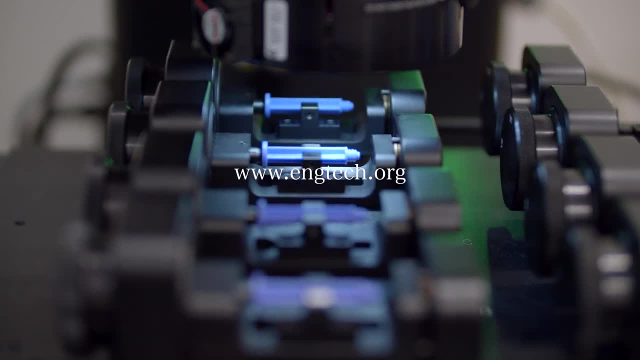 ET programs across the country would be very interested to talk to you and give you more information. We're here for you.